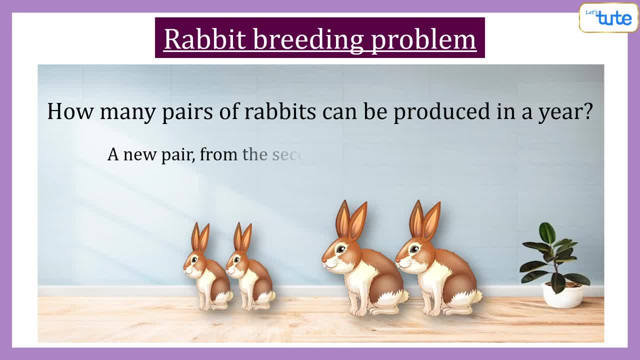 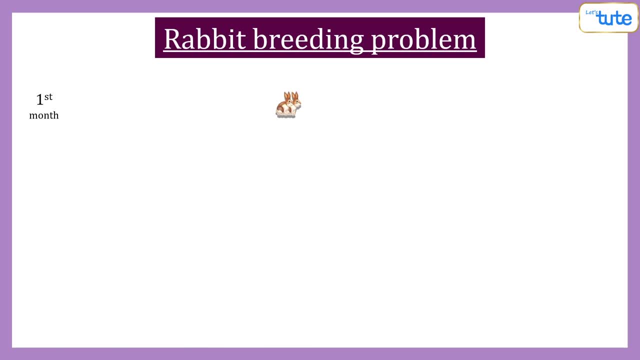 every month, each pair begets a new pair which, from the second month on, become productive. Let's first understand and try to solve this problem. In the first month we had only one pair of rabbits. In the second month this pair will produce one pair of offspring, Then the first. 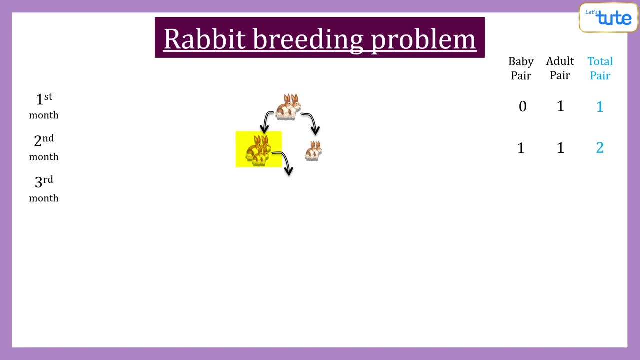 pair will have another pair of offspring in the third month, and the second pair is now mature. Thus, in the third month we have one pair of baby rabbits and two pairs of adult rabbits. Next, two mature pairs will give two pairs of offspring in the fourth month, and the baby pair will be 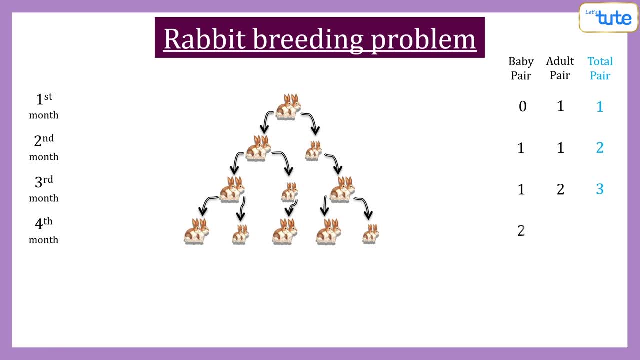 matured now. So there will be two baby pair rabbits and three mature pairs of rabbits in the fourth month. We get five mature rabbits in the fifth month, and each of the three that matured in the previous month has contributed a baby pair. The three previously immature ones will have matured. 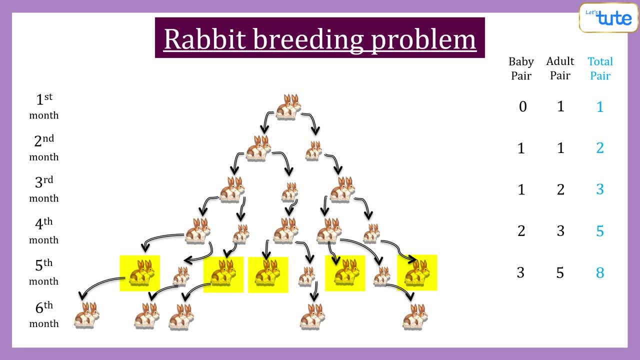 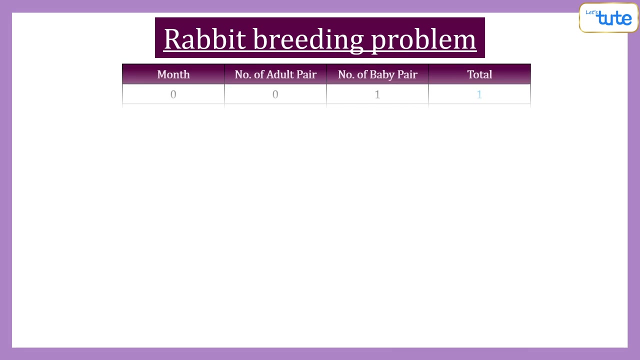 and can be added to the previous five in the sixth month. Thus, we have eight mature pairs and five pairs of baby rabbits in the sixth month. Do you see the pattern? Each new number is obtained by adding the previous two numbers, So let us continue. 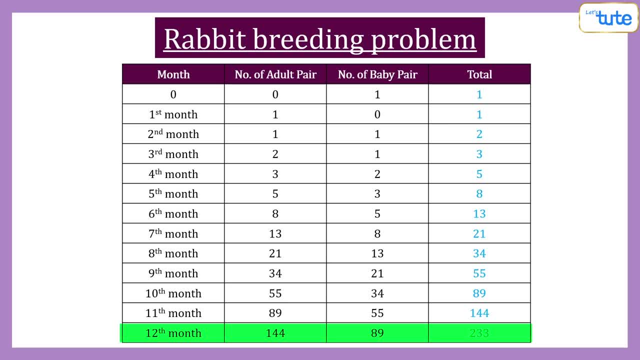 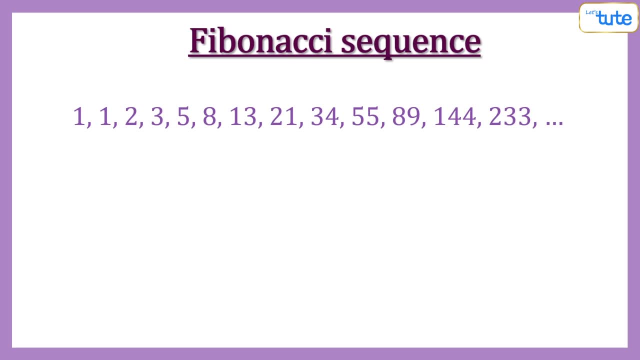 this pattern until the 12th month. So there will be total 233 pairs of rabbits at the end of the year. Do you know what this pattern is called? This pattern is called the Fibonacci sequence, in which the next number is found by adding the previous two numbers. But why? 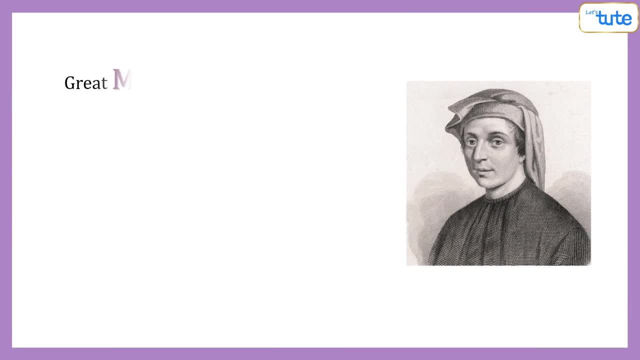 the name Fibonacci. Well, Fibonacci was a great mathematician. around 800 years ago He wrote a book called Liber Abasi in which he asked about this question: the rabbit braiding problem. Do you know? his real name was Leonardo the pizza, and Fibonacci is his nickname. So